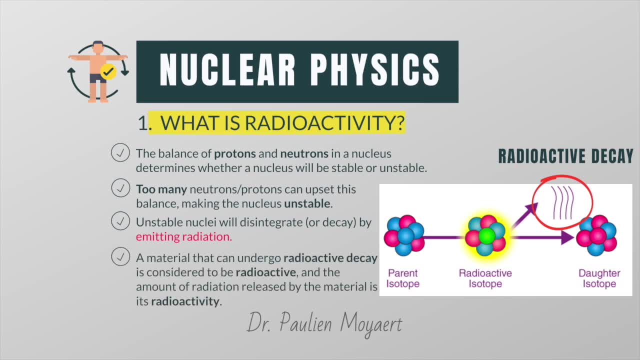 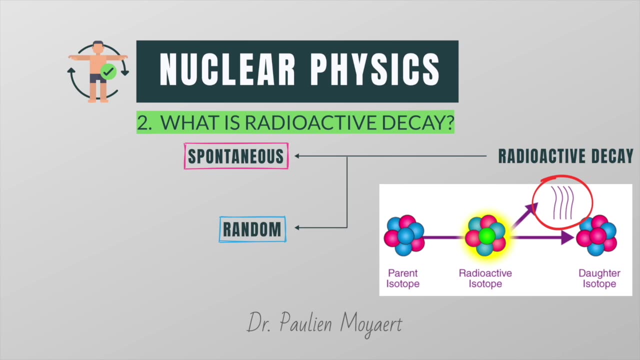 A material that can undergo radioactive decay is considered to be radioactive, and the amount of radiation released by the material is its radioactivity. Radioactive decay is a spontaneous and random process. It means that it is not possible to say which particular nucleus from a block of radioactive 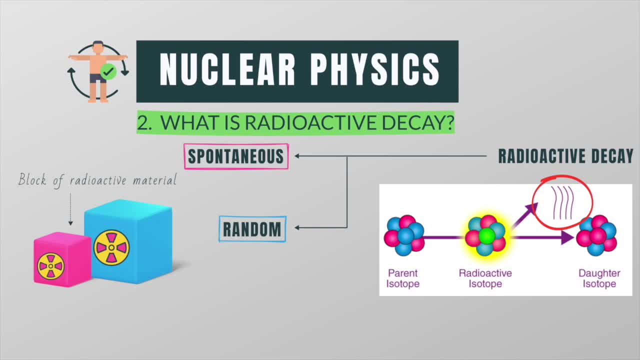 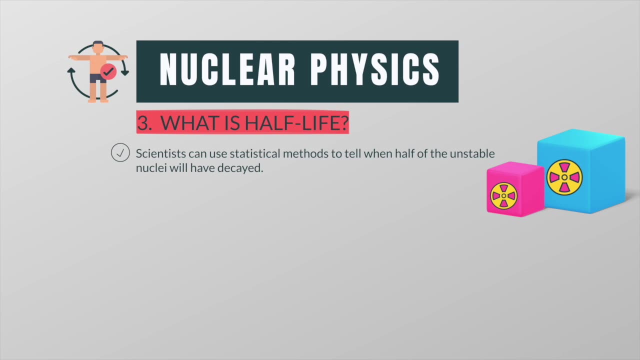 material will decay next, But given that there are so many of them, it is possible to say that a certain number will decay in a certain time. Scientists can use statistical methods to tell when half of the unstable nuclei will have decayed. This is called the half-life. 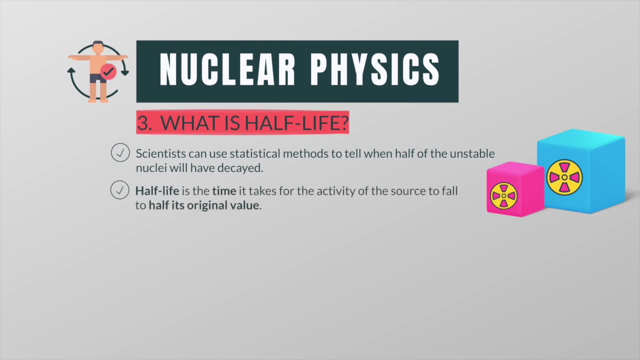 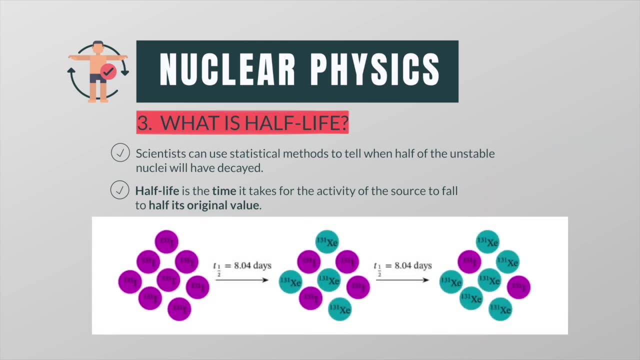 Half-life is the time it takes for the activity of the source to fall to half its original value. Here is an example of how a radioactive sample is decaying over time. Iodine 131 is a radioactive isotope of iodine that is commonly used to treat hypertension. 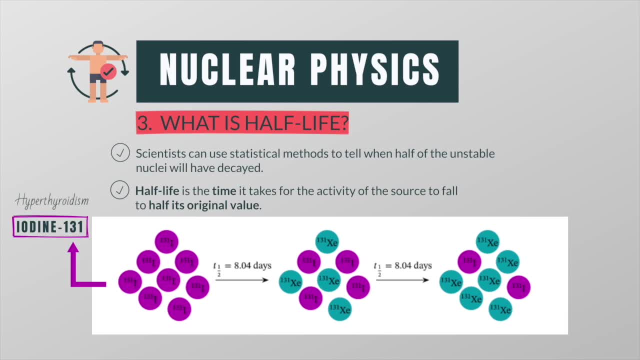 Iodine 131 undergoes beta decay to become stable xenon 131.. The half-life of this reaction is approximately 8 days. This means that if we had a sample of 8 iodine atoms after 8 days, half of the atoms will 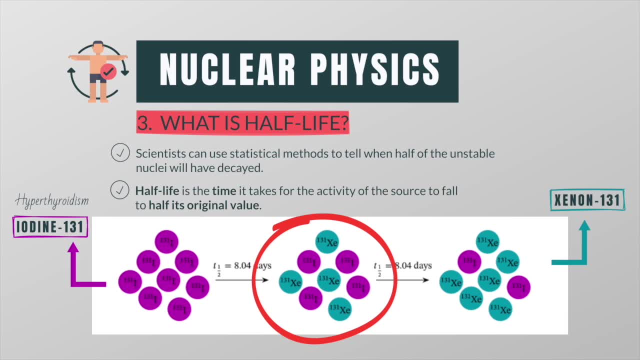 have decayed to form xenon and half of the atoms will still be radioactive iodine. After an additional 8 days, half of the still radioactive iodine will decay. This means that if we had a sample of 8 iodine atoms, after 8 days, half of the atoms will 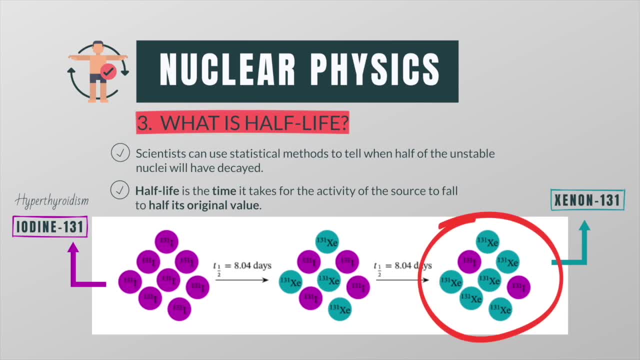 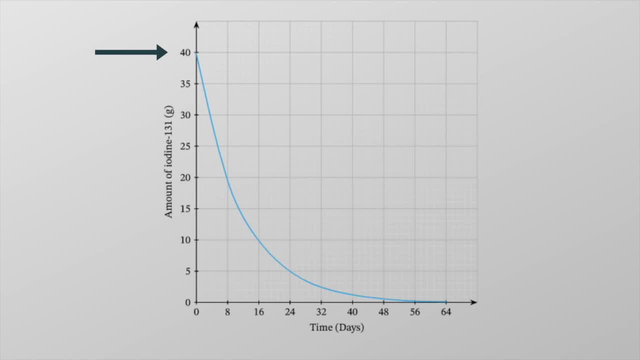 decay, leaving 2 atoms of iodine. This same idea would apply if we measured our sample in grams instead of atoms. If we started with 40 grams of iodine after one half-life or 8 days, 20 grams would have. 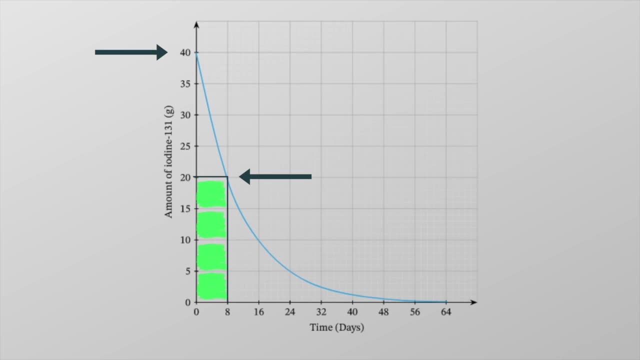 decayed into xenon and 20 grams would still be radioactive After an additional half-life. 10 grams of the original sample would still be iodine, while the remaining 30 grams would still be radioactive iodine. The same idea would apply if we measured our sample in grams instead of atoms. 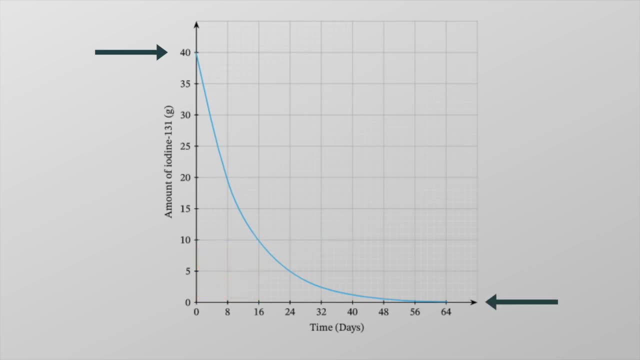 When the total amount of iodine has become growing up. the original sample would have decayed into xenon lasse to 0 and w Xia to 0. Note that this process continues and although the amount of iodine might get very small, it does not drop to zero completely.